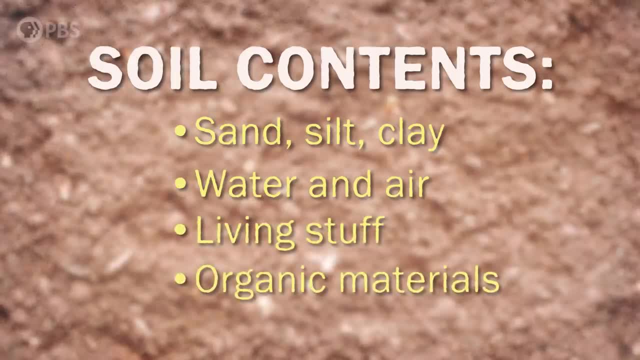 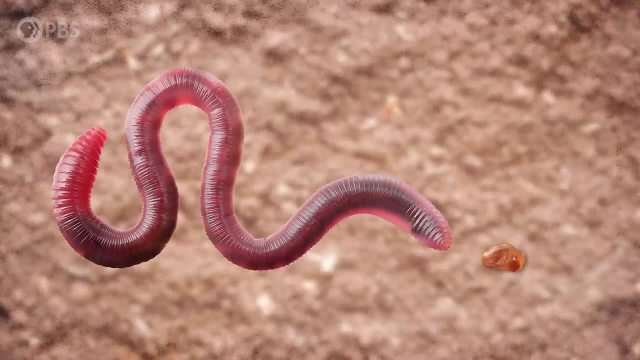 stuff and also formerly living stuff that is decomposing, adding organic material into the soil. All of these components of soil are different sizes, from the comparatively massive earthworm to the large particles of sand, down to the teensy pieces of clay and the minuscule bacteria. 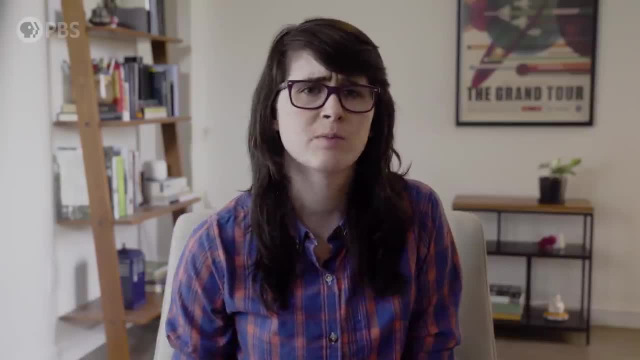 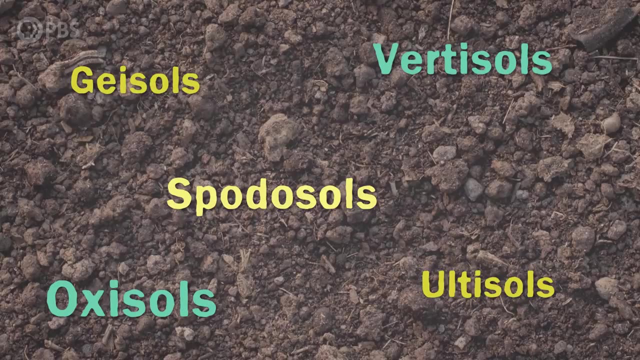 And maybe obviously not all soil is the same. You might live somewhere with really sandy soil, or a place with distinct layers or lots of rocks, But regardless, all these different soils with funny names are still soil. To get a better understanding of the diversity of all these different types of soil, we're 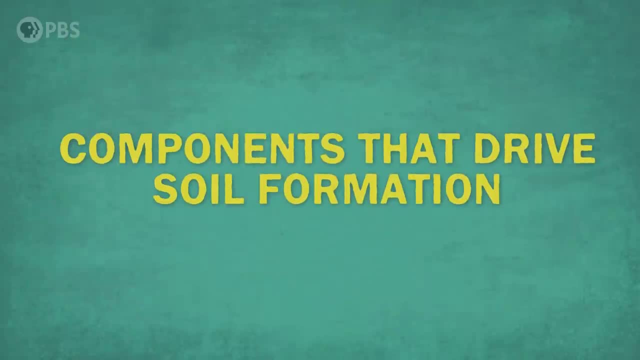 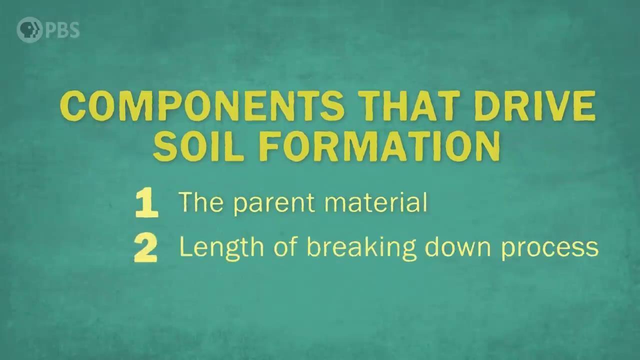 going to look at the five main components that drive soil formation. 1. The parent material: The type of rock that, over a really, really, really, really really long time, broke down. 2. How long that breaking down process took. 3. The types of organisms living in the soil. 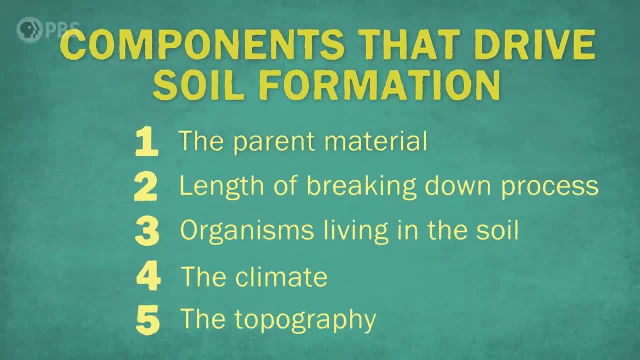 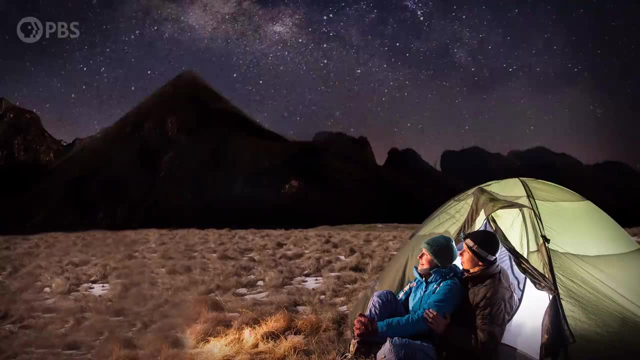 4. The climate of the place the soil is in. 5. The topography of the area. Let's dig into that list a bit, shall we? Soil doesn't just appear out of nowhere, So let's imagine for a moment that we're. 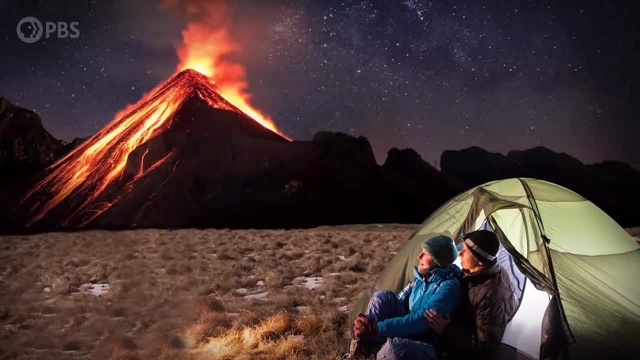 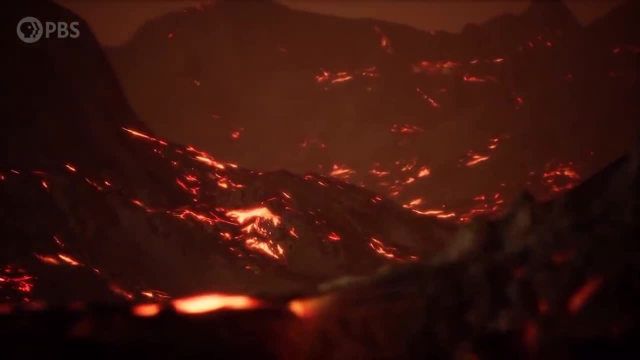 hanging out just minding our own business, and we see a volcano erupt. We're safe, but we see a little landslide of lava. It completely burns and covers whatever was there before. So there isn't any soil now, But if we hit fast forward, the soil will come. 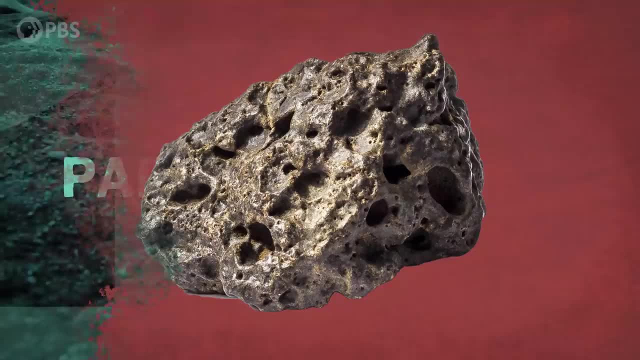 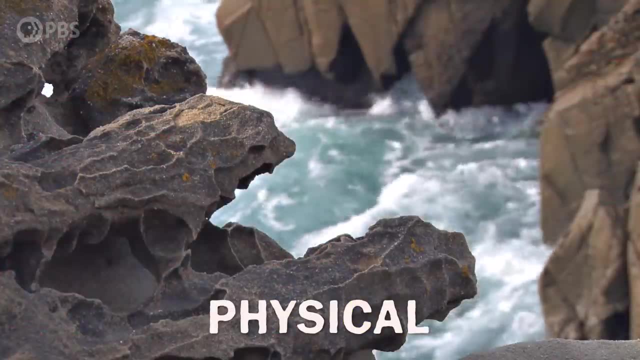 back. It starts with the parent material, In this case volcanic rock. Over time, that rock will slowly break up into loads of tiny pieces through a process called the process of breaking down. This could be physical, like wind or water smashing into the rock and breaking off bits. 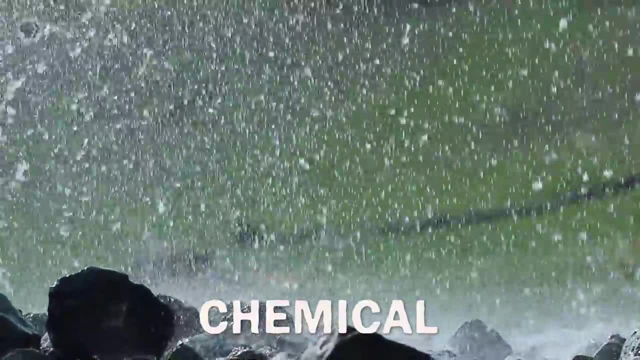 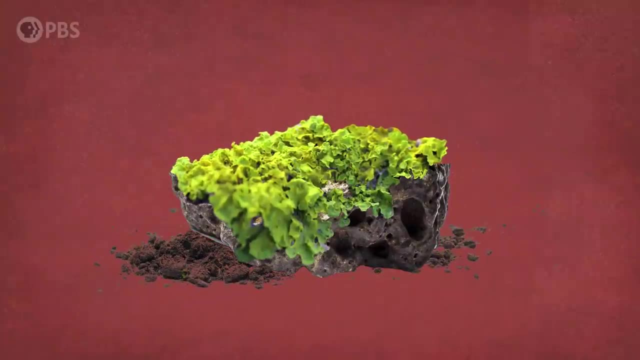 or it could be chemical: the rock particles interacting with material in the air or water, like acid rain, or pioneer species. Pioneer species like lichen can hop on our lava rock and secrete an acid that breaks down the parent material. Pioneer species- lichen or bacteria- are all our selected species, meaning they have a 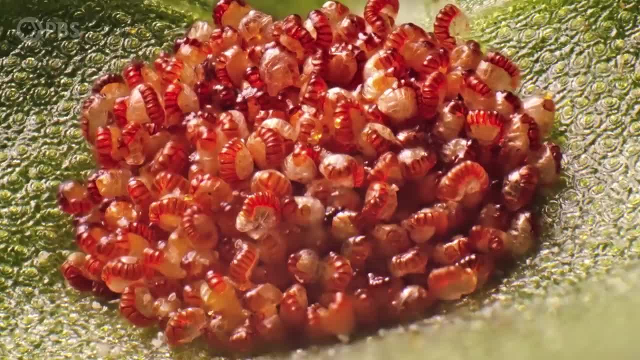 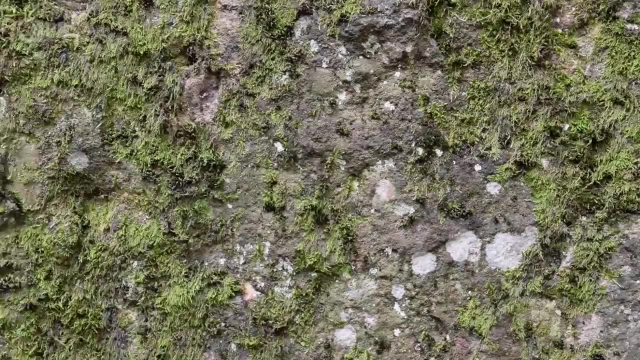 high reproductive rate and will crank out lots of little offspring and babies, and spores and seeds, knowing that the majority of them will not make it in this harsh habitat. but the ones that do will grow and thrive. Eventually, these pioneer species are going to die And when they die, they're going. 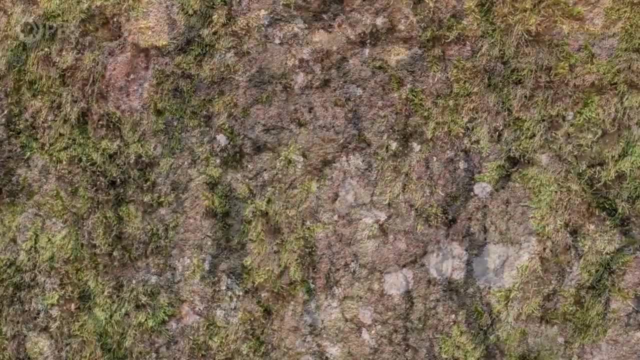 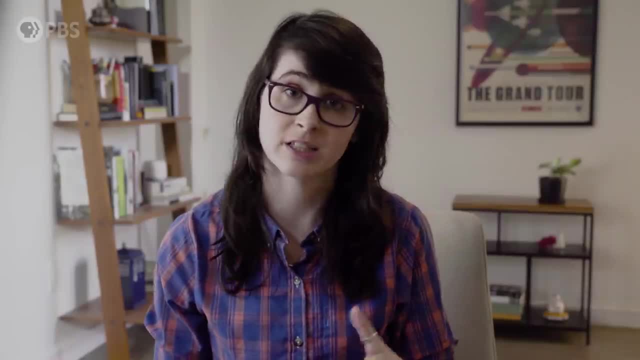 to decompose and their decomposed tissues are going to go into the weathered pieces of rock. And now this mixture is soil. The broken down parent material is the base of the soil And, kind of like a baby, inherits characteristics from their parents. soil inherits characteristics from its parent material. 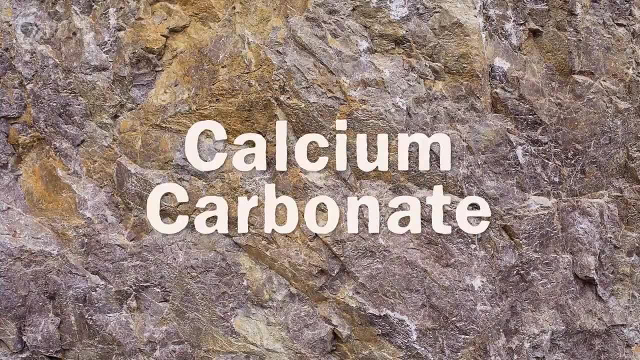 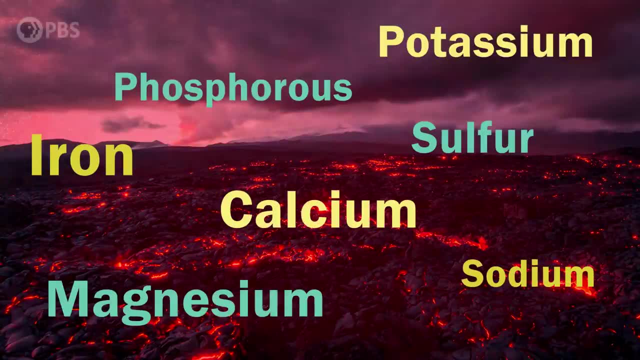 For example, limestone is a rock that's rich in calcium carbonate, so the soil that results from limestone rock has typically a lot of calcium in it, Or in our lava field, it contains a bunch of different nutrients because it's made up of materials pulled. 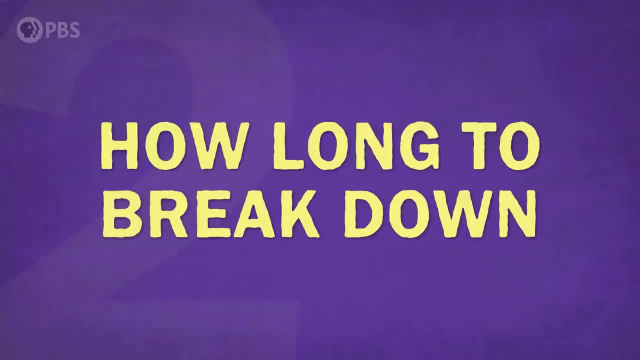 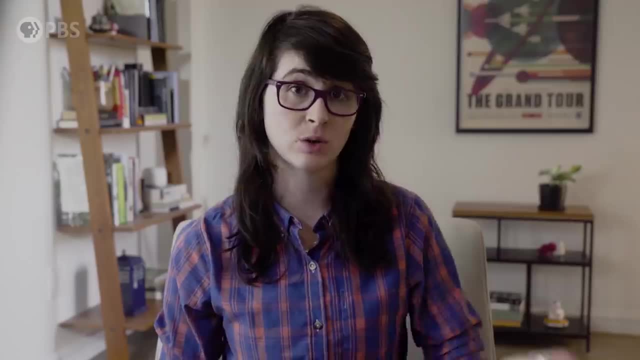 from deep underground. This obviously takes a long time. Rocks are pretty hard, so breaking them down is a whole process, which is why time really matters in classifying soil types. As soil goes from young and immature to mature and robust, the living community on top of the soil gets bigger. and more complex along with the soil. Over time, mature soil with distinct layers forms And, like magic, and over a few hundred years, our barren lava field will transform to a forest. In addition to the parent material and the age of the soil, we've got to look at what. 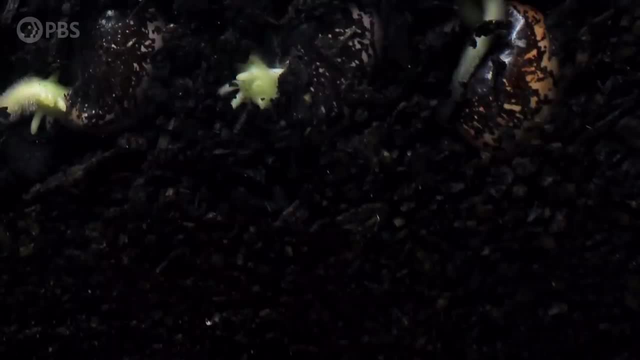 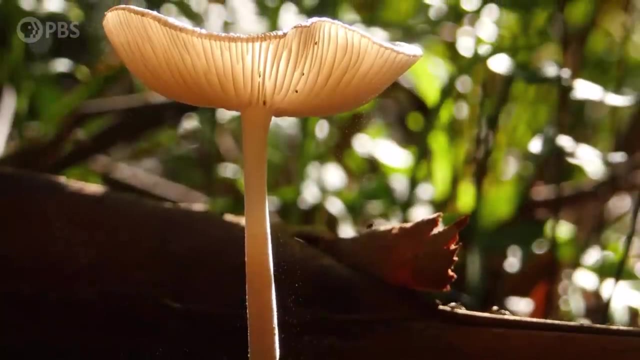 organisms are hanging out in and on it. There are a lot of living things in soil, Like a lot. More than a million microorganisms live in a single teaspoon of fertile soil. There are microorganisms and worms and moles and gophers and plants and fungi. Those plants 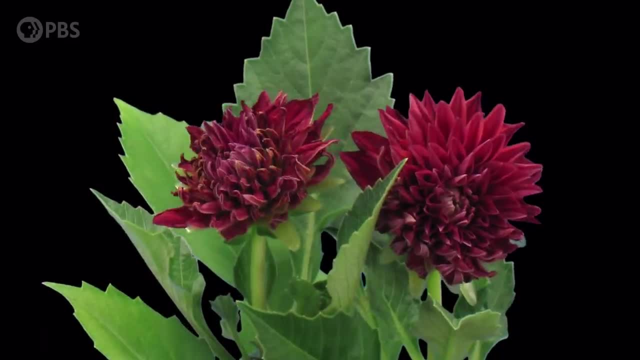 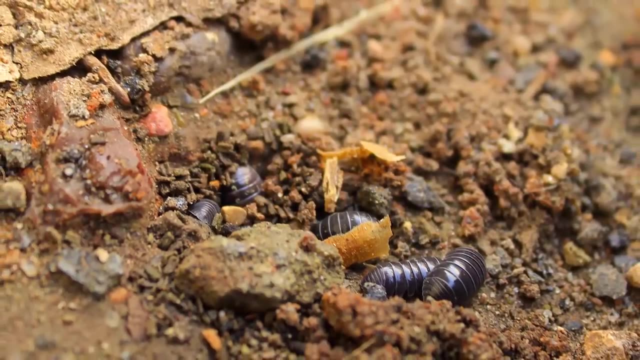 are taking nutrients out of the soil, But when they die and decompose they'll bring it right back in. And all those animals and plants squirming around aerates and mixes the soil, This combination of living and dying organisms all mixed up with the parent material. 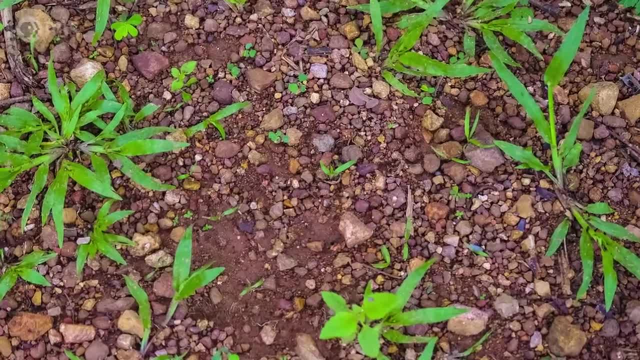 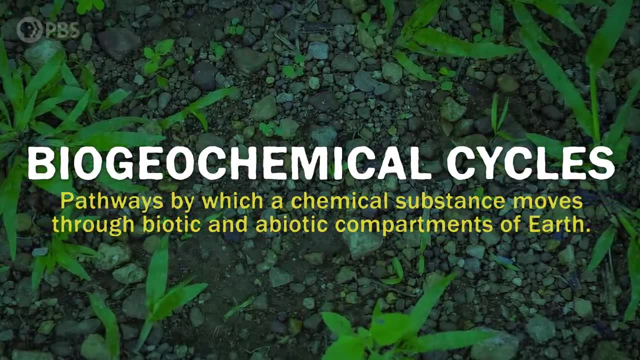 minerals and nutrients is what makes soil such a key component of the biogeochemical cycles of our planet, Which means soil plays a major part in how nutrients and minerals flow through the biosphere. So let's take a look at one part of one of those processes. This is a rough cartoon. 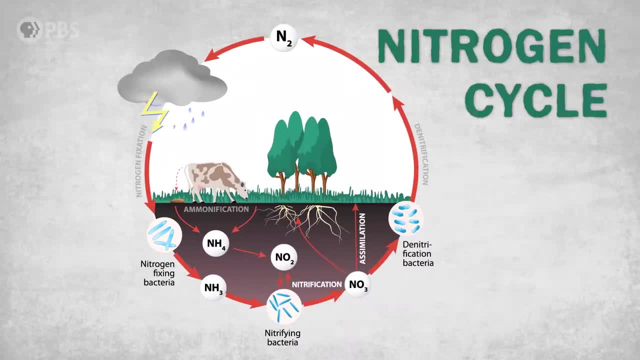 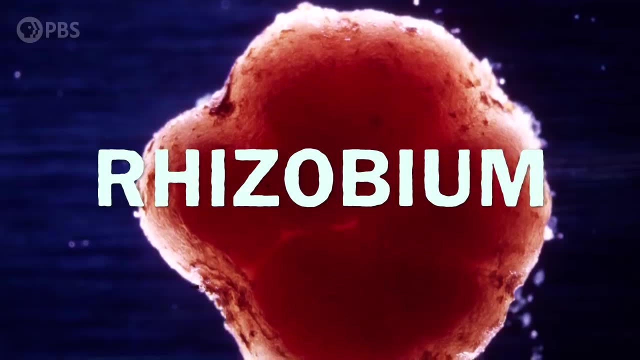 of the nitrogen cycle. Nitrogen is pretty important for plants because they need it for photosynthesis. But the nitrogen gas in the air plants can't use. It's in the wrong shape. Enter rhizobium, This little bacterium. well, all bacteria a little. but 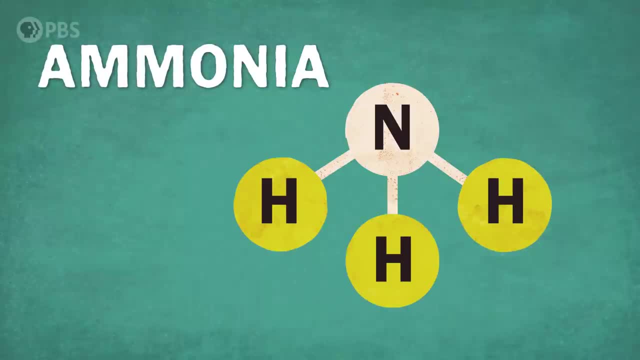 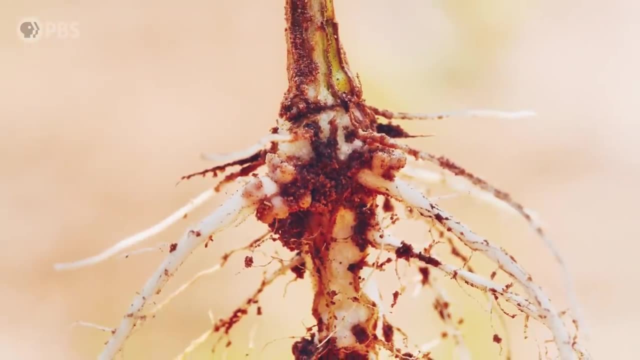 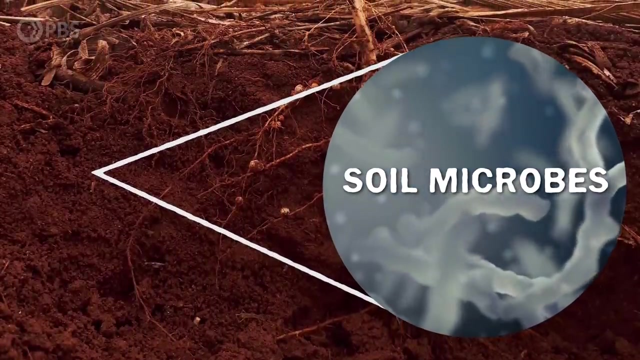 this one has the incredible ability to turn atmospheric nitrogen into ammonia. Ammonia is the form of nitrogen that plants love. Rhizobium basically gives the plants its own microscopic fertilizer factory, converting unusable nitrogen into a form usable by the plant- all in the soil beneath our feet. And rhizobium isn't alone: The nitrogen cycle. 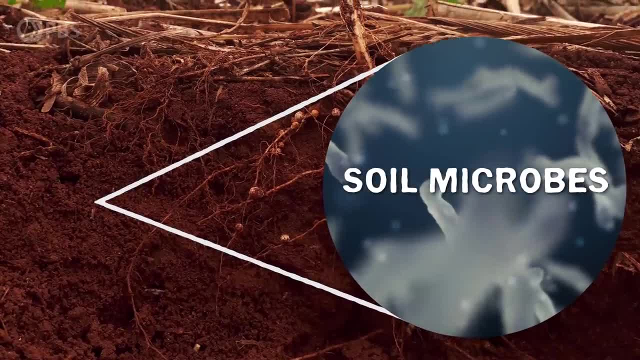 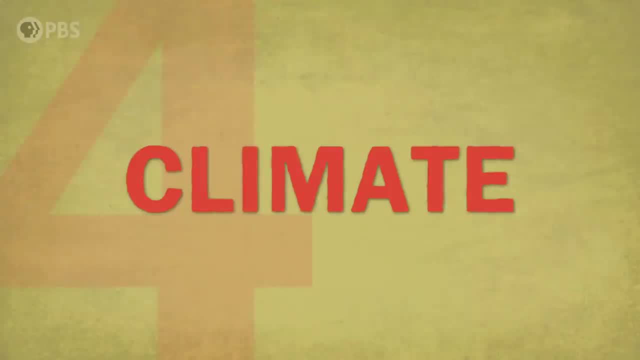 the carbon cycle. basically all nutrient cycling between the abiotic and biotic parts of our planet is driven by these soil microbes. Climate's influence on soil formation is pretty varied depending on where you are on Earth. Inflammation and humidity are some of the big factors, Super cold temperatures, or really. 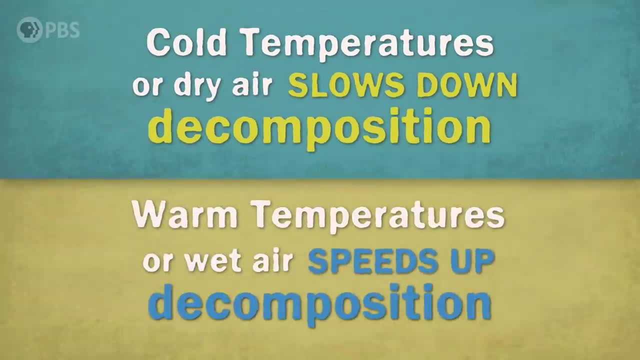 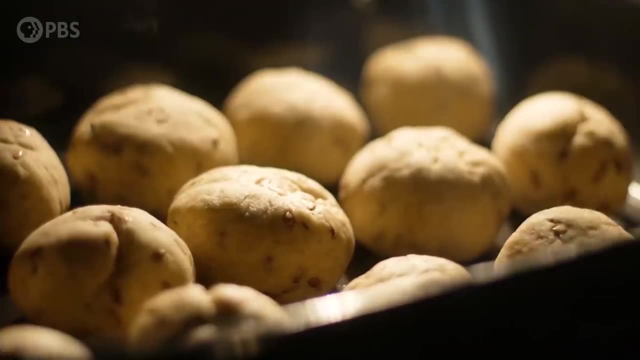 dry air will slow down decomposition. Conversely, warm and wet conditions will speed up decomposition and soil formation. Think a frozen tundra versus a rainforest, Or how, when you're cooking in the kitchen, you can start with the same ingredients and get a different meal. 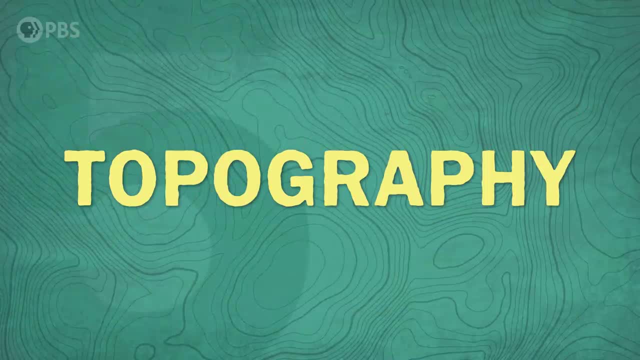 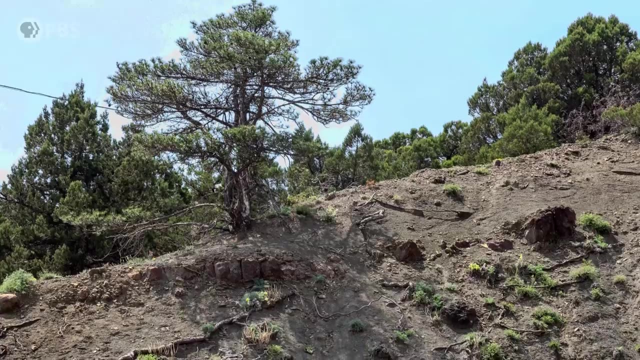 depending on how you cook them. And finally, topography will also influence soil formation. Topography is the landforms and landscapes of an area. Is it hilly or flat or full of canyons? Something with a steep slope might result in high erosion. 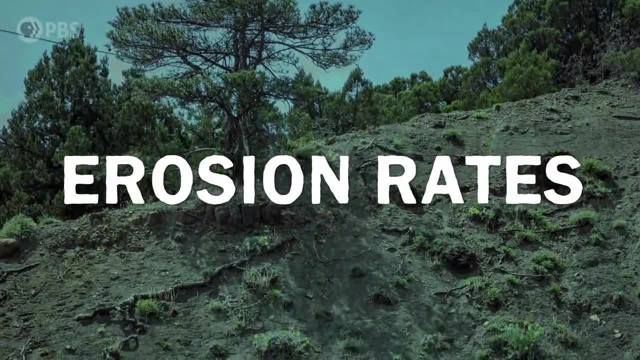 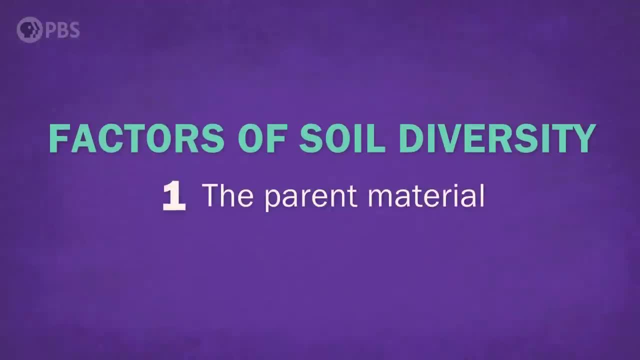 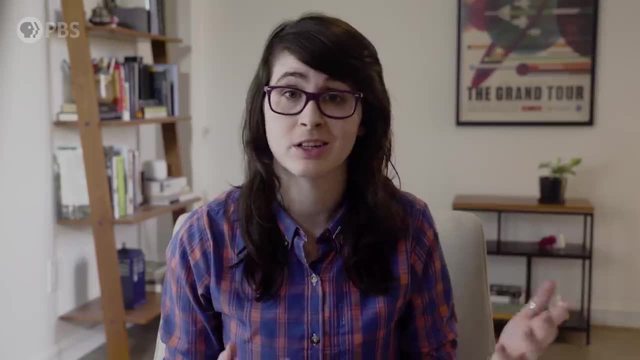 And a loose, dusty soil, whereas thicker soils might form down in the valley between two mountains. These are the five factors that create the diversity of soil: Parent material, time, organisms, climate and topography. But so what? Why do we care that there's these different types of soil? Well, because 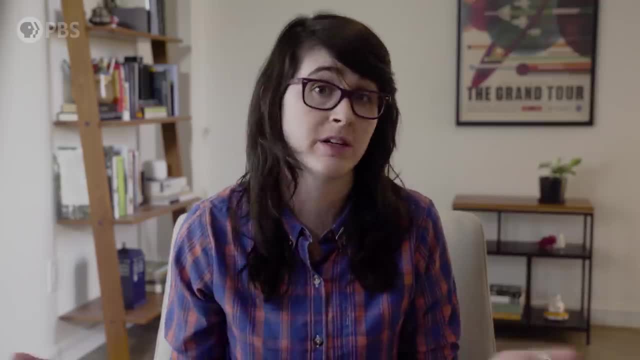 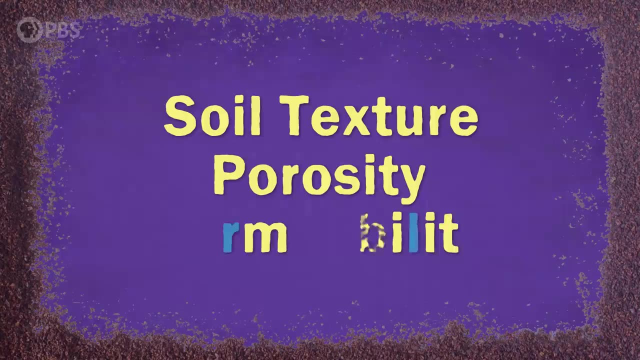 each type does different things and we and other species use them differently, And that all comes down to the soil's properties. We'll start with the physical properties: soil texture, porosity and permeability. Soil texture is determined by the percentage of soil that is produced by the soil. Soil's. 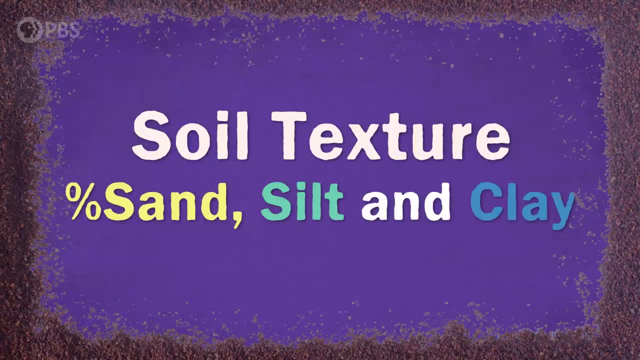 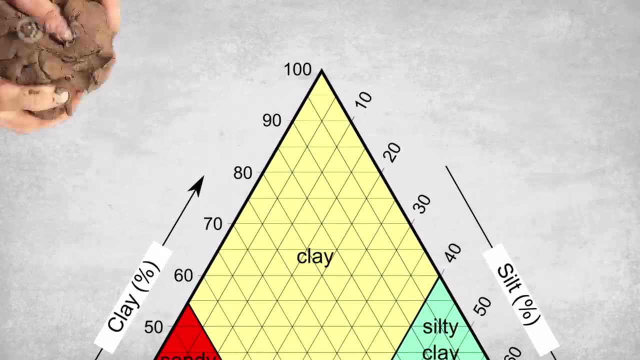 percentage is the percentage of sand, silt and clay, Those weathered down tiny pieces of rock that make up the soil. Scientists use the soil triangle as a way to represent soil texture. Up here at the top of the triangle, that's 100% clay. Great for making pottery Over here. 100% sand. 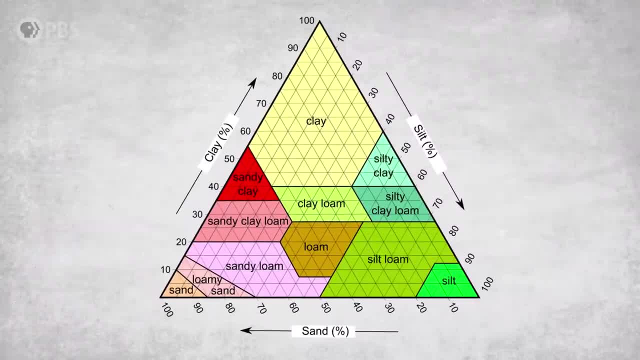 Great for making castles. But most soils are a combination of all three- Sand, silt and clay- So we can triangulate the kind of soil we have. 21% clay would be along this line, 66% sand would be right here and then 13% silt would be here. So this particular type of 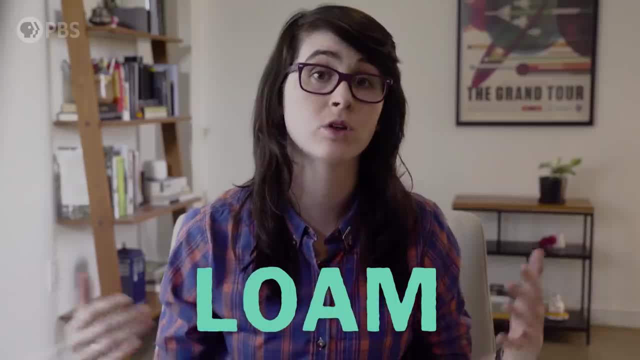 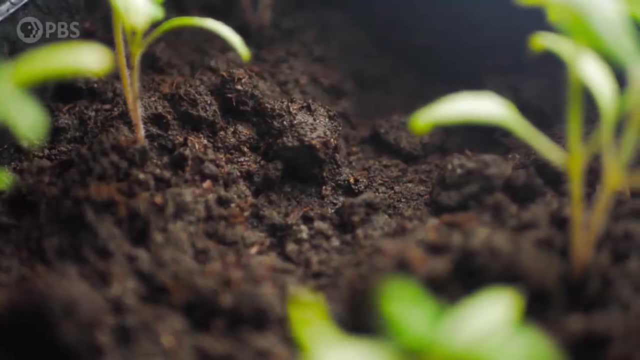 soil with those percentages is called soil texture. Soil texture is a combination of sand, silt and clay, And the word loam is important. Loamy soils are like Little Bear's porridge for Goldilocks: Not too hot or too cold, It's just right. Loamy soil is just. 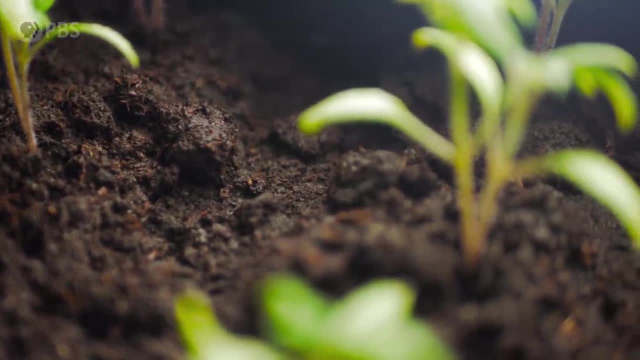 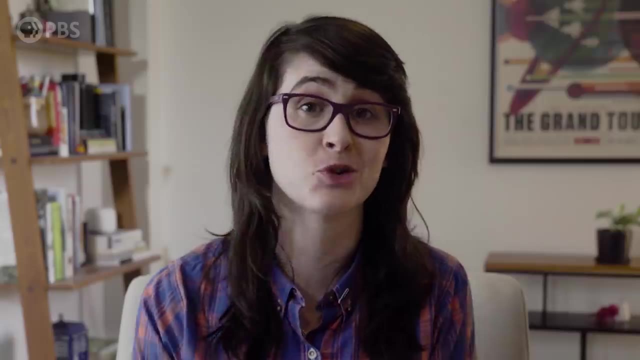 the right mix of sand, silt and clay to be beneficial for agricultural uses. And here's where we point out what might be really obvious to you: The vast majority of our caloric intake comes from things that are grown in the soil. 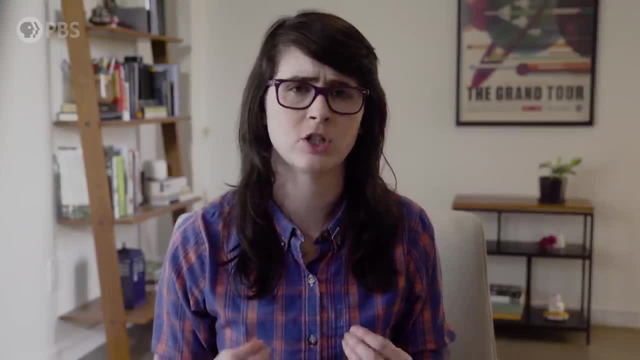 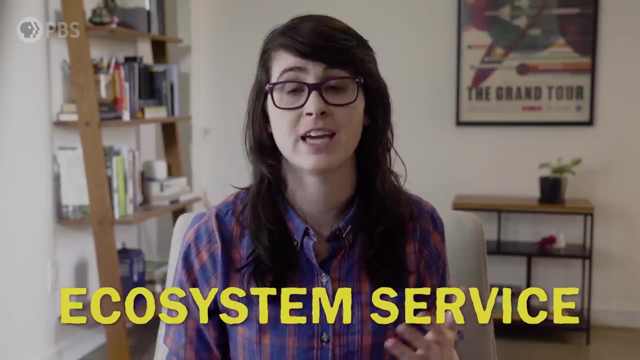 Just like we learned in the water lesson that preserving ecosystems and watersheds is a cheaper and more effective way to clean up drinking water, we rely on soil as an ecosystem purpose Because it's a fundamental component of the agricultural system. we use every single. 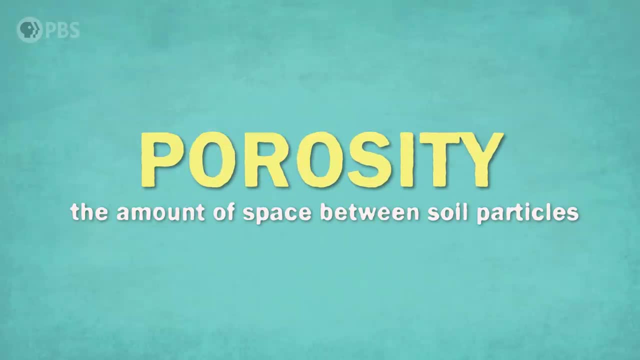 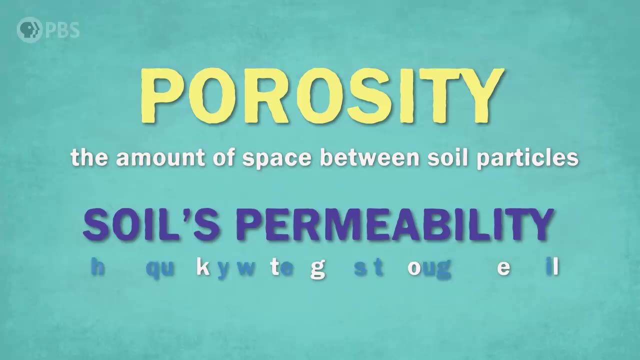 day. The next physical property: Porosity. This is simply the amount of space between the soil particles that determines how much water and air can move through the soil, Which is related to the soil's permeability. How quickly will water go through the soil? 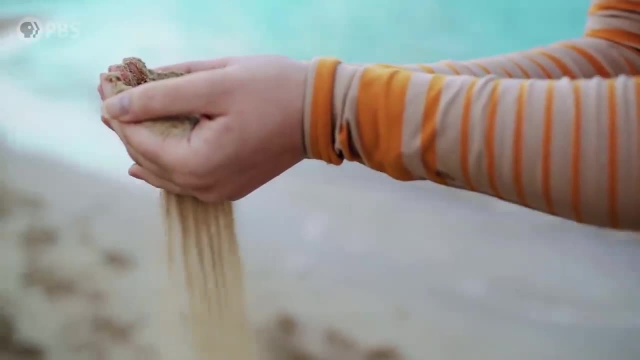 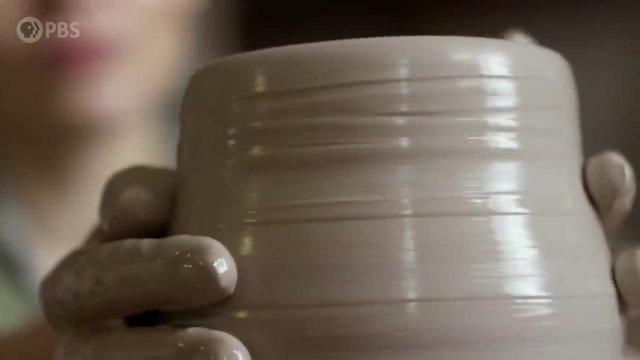 Sand is more permeable than clay, so imagine if you had a handful of sand and you poured some water through it. Most of the water would just pass right through, as opposed to clay, which will actually hold the water in. That's why pottery works. 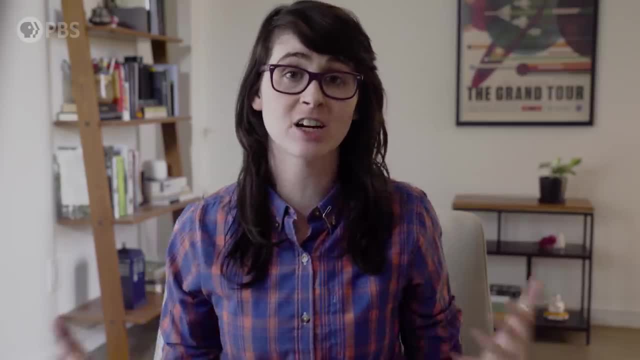 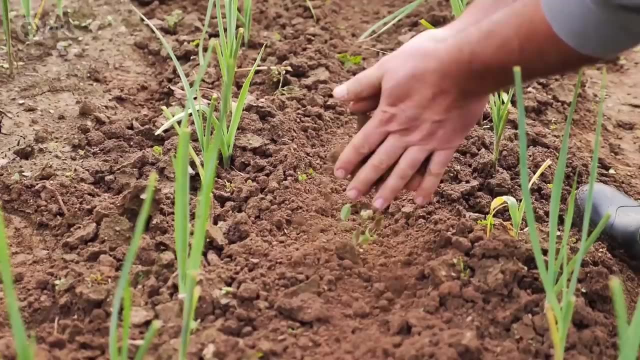 If we combine what we know about soil texture, porosity and permeability, we can start to get an idea of what different types of soil can do and be useful for When farmers are planning and taking care of their crops. identifying the soil's physical 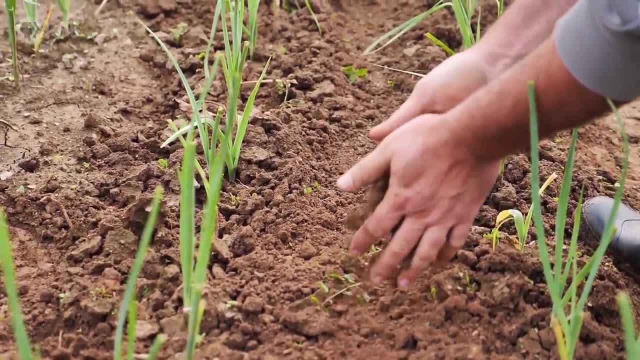 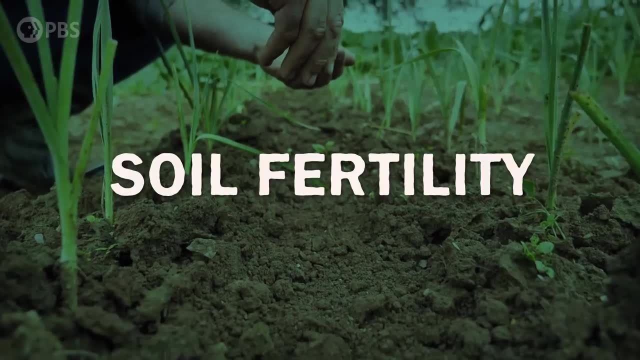 properties is a big part of making sure they irrigate or water their plants and soil appropriately. Farmers also need to consider the chemical properties of their soil, like soil fertility, As we talked about. plants need certain nutrients to grow and ideally, these are going to come. 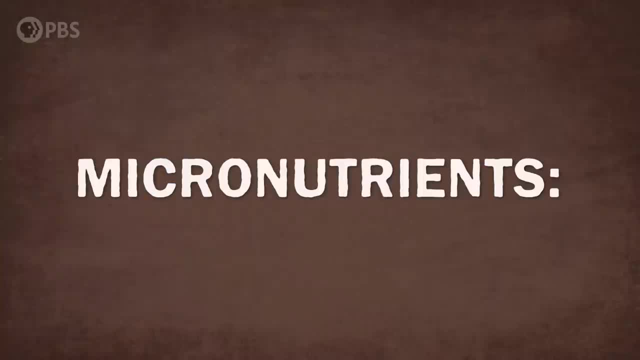 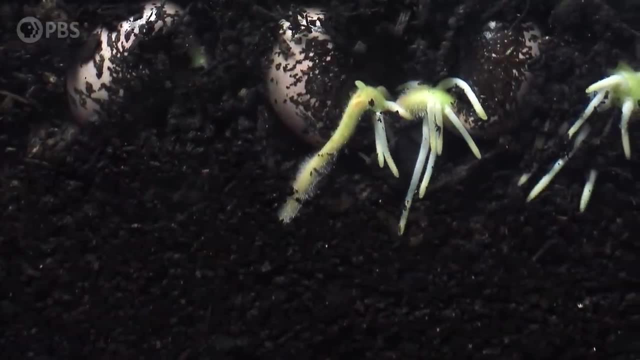 from well balanced soil. This balance of micronutrients like nitrogen, but also phosphors and potassium, is the soil's fertility, And those micronutrients and other organic matter the plants crave largely comes from the chemical properties of the parent material of the soil as well. 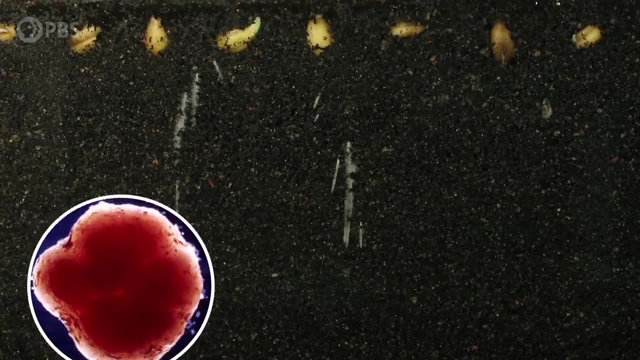 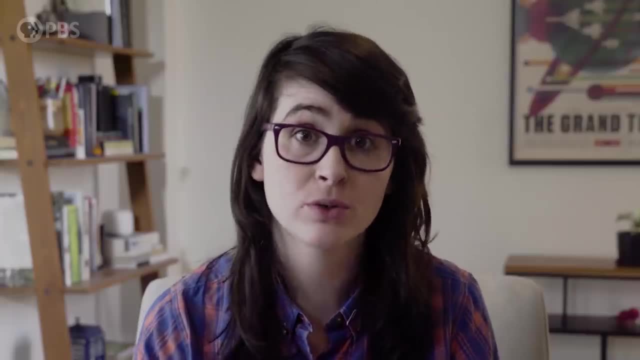 as the organisms, like our rhizobium, living in the soil, When well-managed soils with high fertility can support abundant, healthy plant life. But I don't want to just talk about the benefits of healthy soil for our food system. 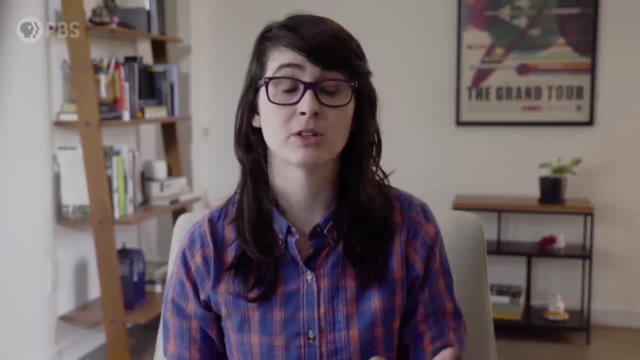 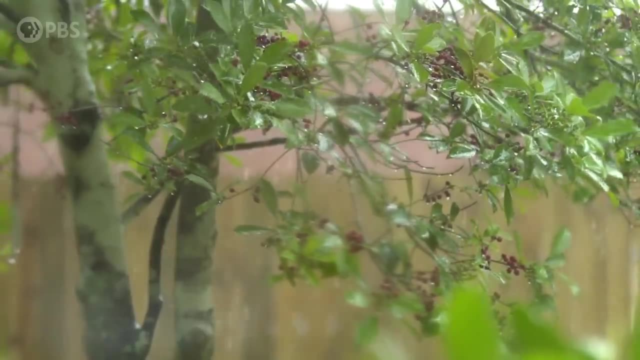 The ecosystem services that soils provides are so much bigger. Remember, soil is everywhere. It's the top layer of earth and we rely on it for a lot of things underground, Especially groundwater. Soil is a fantastic filter After a rainstorm water which could have. 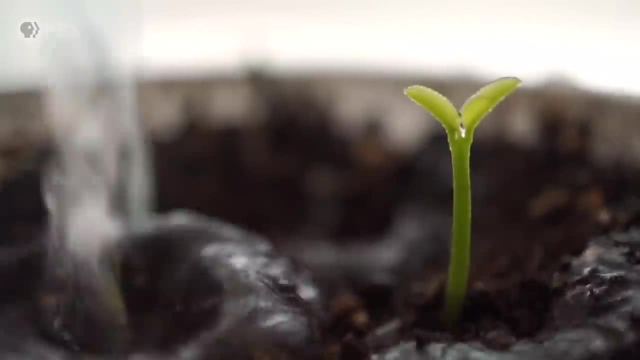 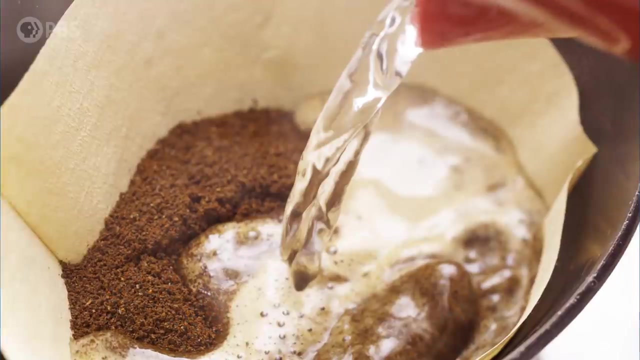 picked up who knows what in the atmosphere or some gross stuff on the ground, slowly makes its way downward, heading toward an aquifer, an underground body of water. But to get to that aquifer, all along the way, like a bajillion coffee filters, soil pulls. out the stuff that isn't good to drink, And in some places we barely have to treat our groundwater to make it drinkable because soil does it for us. Soil provides all these incredible benefits for people: filtering water, helping us grow food. 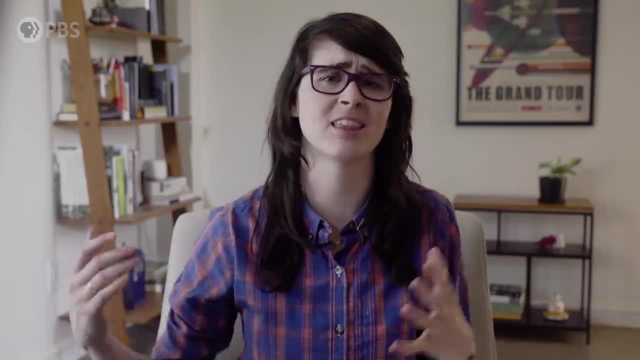 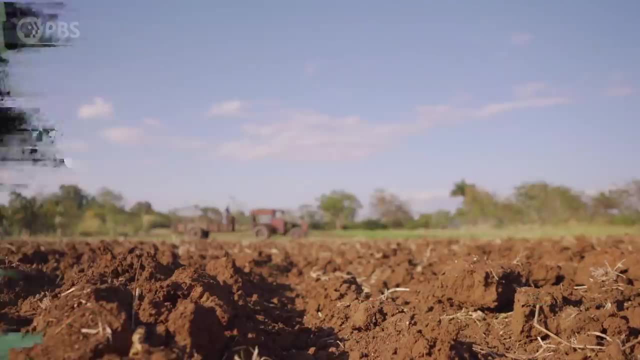 But we don't really have it really return the favor. In fact, human activity is messing up a lot of our great soil out there. Unsustainable agricultural practices can lead to a loss of soil fertility, So things like planting the same thing over and over and over again in the same soil without proper 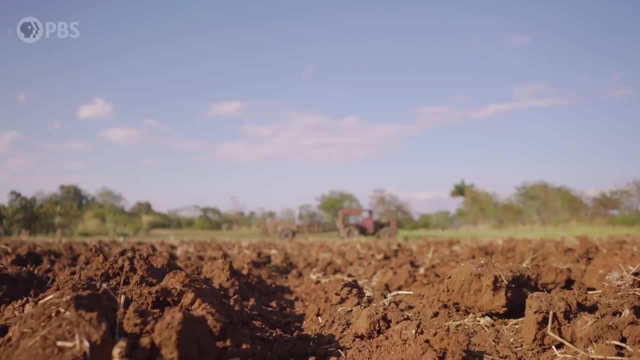 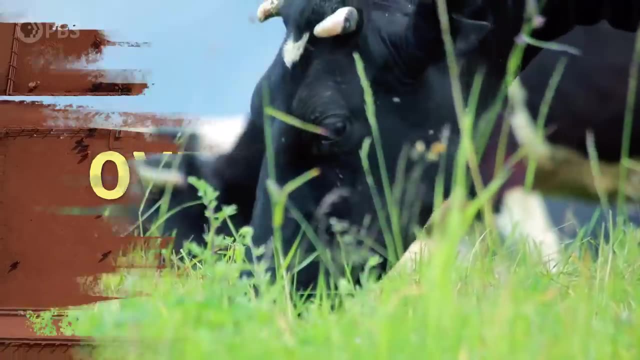 fertilizers and soil management can result in a soil that can no longer support life, Overgrazing when there are too many cattle for an area and they overeat the grasses and compact the soil with their hooves. And once the grasses are all gone, the soil no longer. 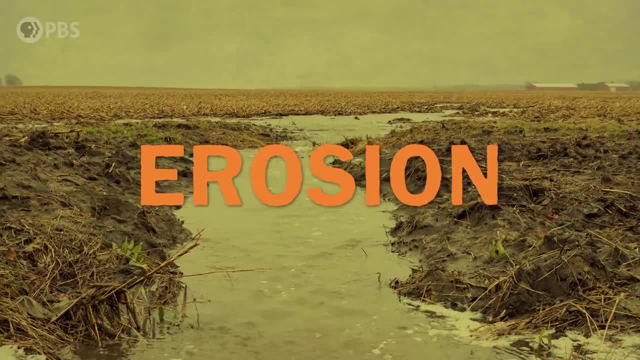 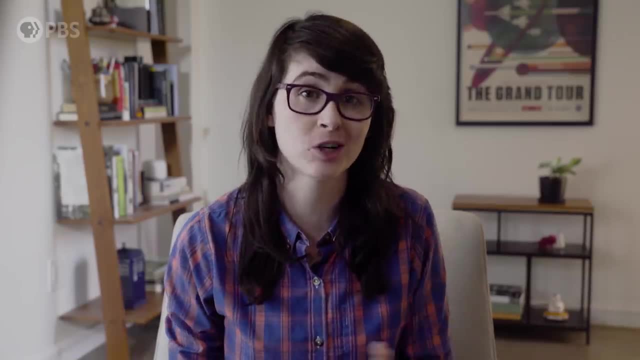 has their roots to hold it in place. So erosion increases and we lose soil. This is a bit heartbreaking because soil takes so long to form from a parent material. Erosion erases millennia of hard work in a matter of days or weeks. 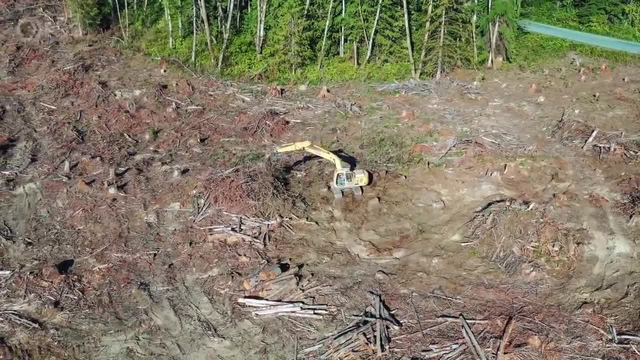 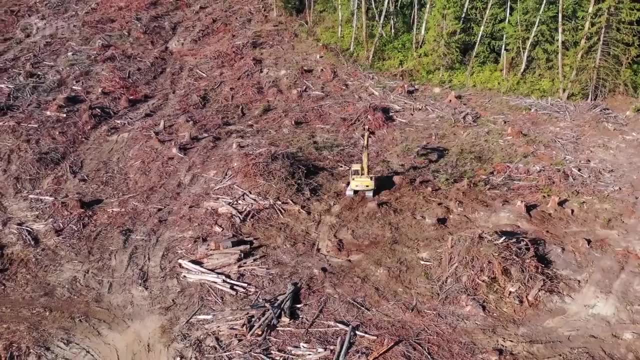 Similarly, deforestation does a real number on soils because by getting rid of these trees with massive root systems that hold a lot of soil in place, suddenly that good, healthy soil supporting an entire forest will just wash away when it rains. This also happens when soil is tilled. Tilling is the process. a lot of folks who grow food 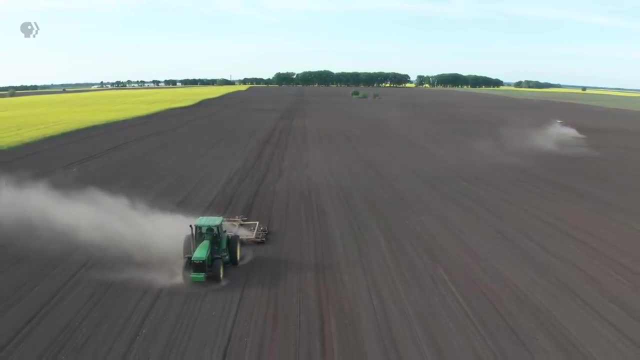 use to grow their crops. This is the process a lot of folks who grow food use to grow their crops. This is the process a lot of folks who grow food use to overturn the soil and get rid of old crops in the preparations for next planting. But this process often leads. 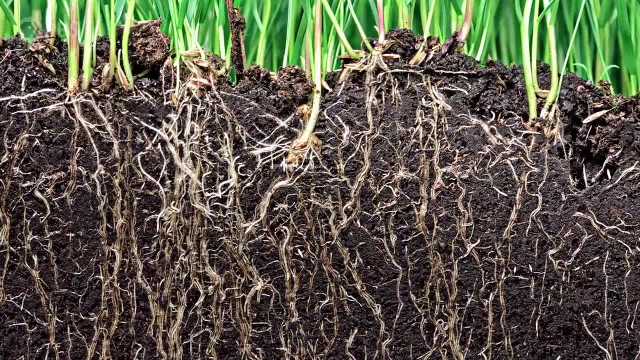 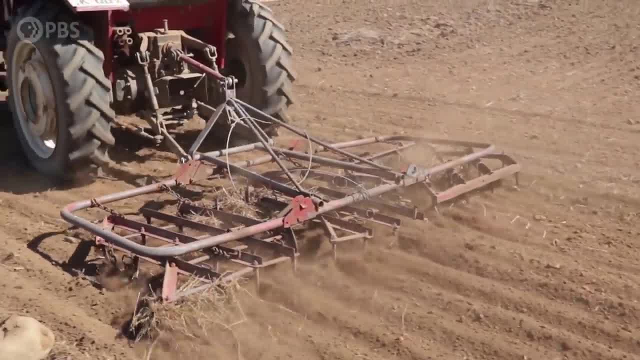 to loads of erosion. Roots, as I've said, are important for soil. Even the old roots from last year's crops matter, And when those rich structures are disturbed and all tossed around during tillage, the wind can easily blow away the soils because they aren't being held together anymore. 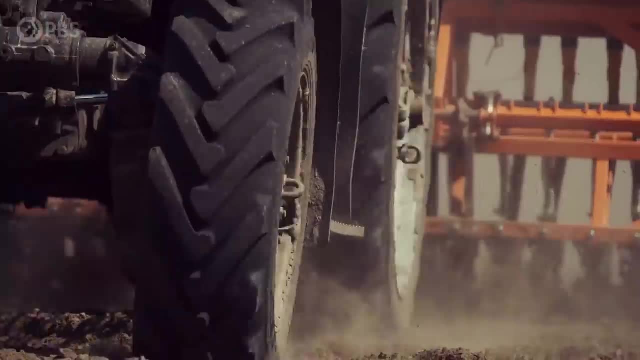 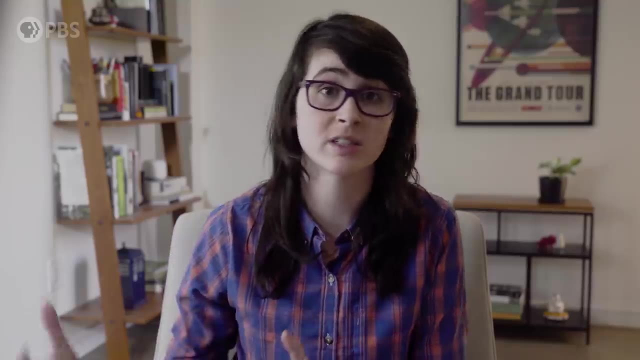 Along the way that soil is also at risk of compaction. All those big tractor tires squishing along the soil can mess up the permeability and the porosity. Unsustainable agriculture: overgrazing, deforestation, overtilling and compaction are all ways human activity. 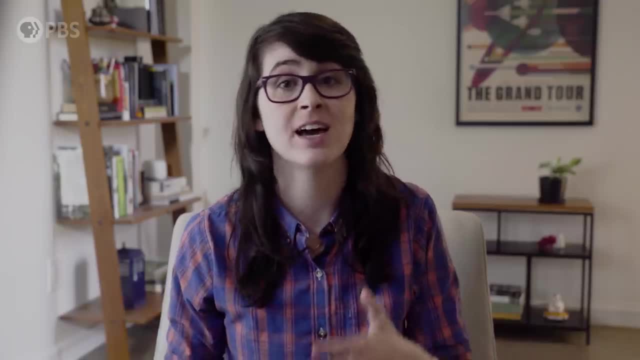 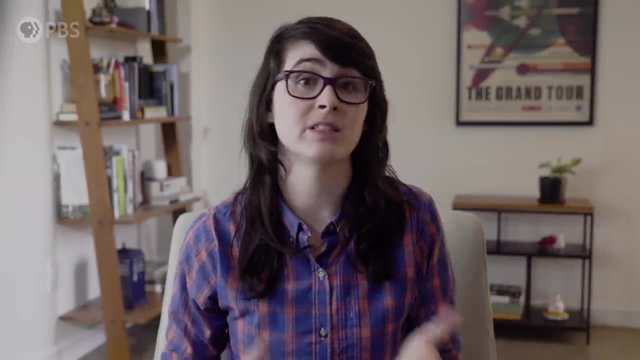 is degrading our soils, reducing agricultural productivity, negatively impacting ecosystems and increasing erosion. But there's one more big reason to protect our soils: Soil is where the air meets the ground, making it a major player in the global climate system. Soil is a carbon sink which 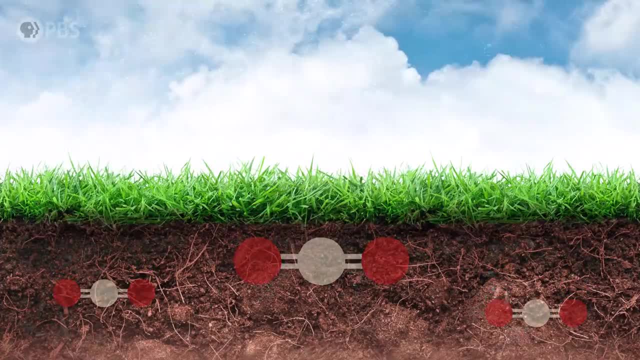 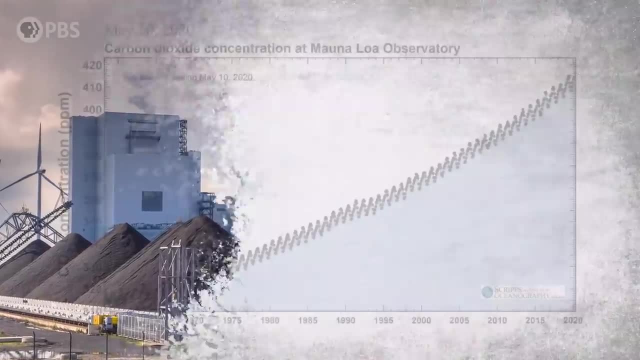 means it can take carbon dioxide from the atmosphere and store it underground, Something that is super needed right now, because we're putting a lot of carbon dioxide into the atmosphere and warming up our soil. This is the famous Keeling Curve, which reports continuous measurements of carbon dioxide. 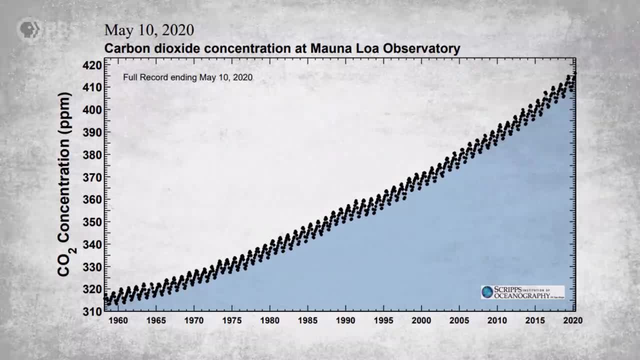 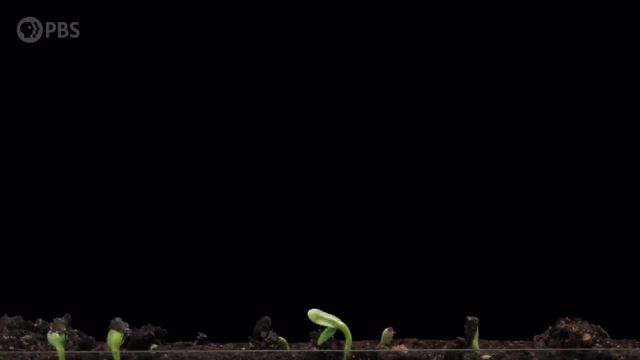 in the air from 1958 to now And we can see that over time, carbon dioxide is increasing. So why is soil a carbon sink? Well, if I'm a plant and I'm doing some photosynthesizing, I'm drawing carbon dioxide out of the air and transforming it into organic compounds. 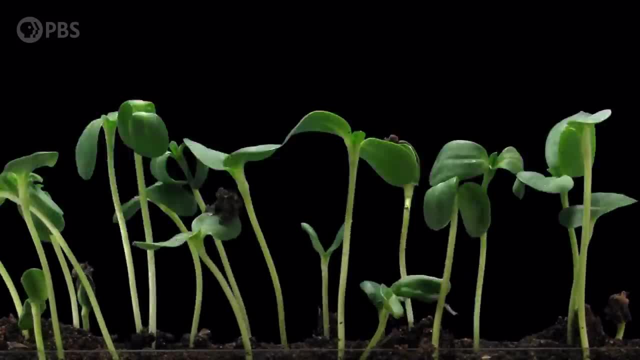 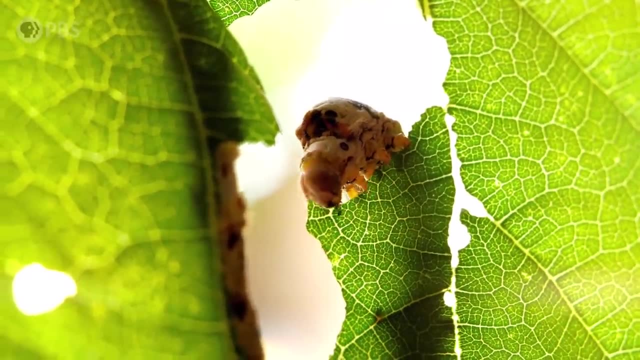 which I store in my little plant body as leaves or kernels of corn or a beautiful flower Or roots. If I get eaten, whatever eats me then turns that carbon into muscle or fur or bone. Eventually plant me and whatever I got turned into is going to die and the